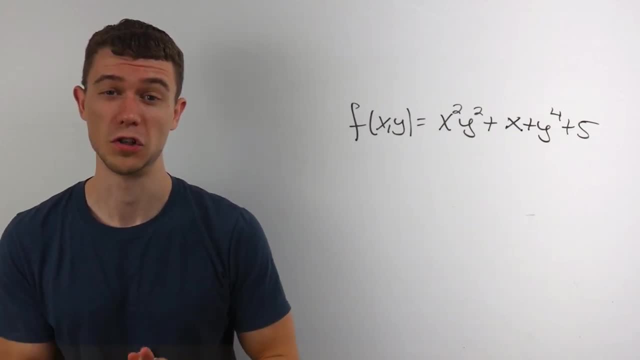 Let's do the partial derivatives of this function. Remember partial derivatives. we only take the derivative with respect to one variable and we treat the other variable as if it is a constant. There's different notations. you might see If this is my function, a function of 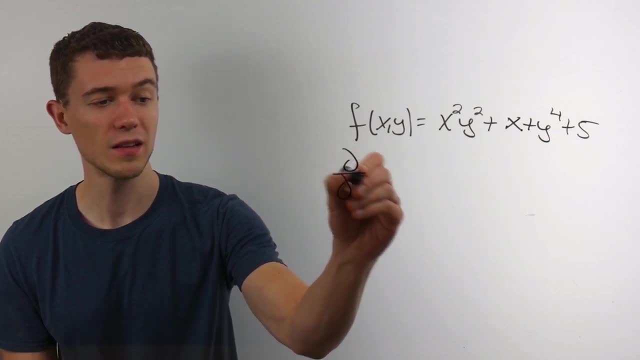 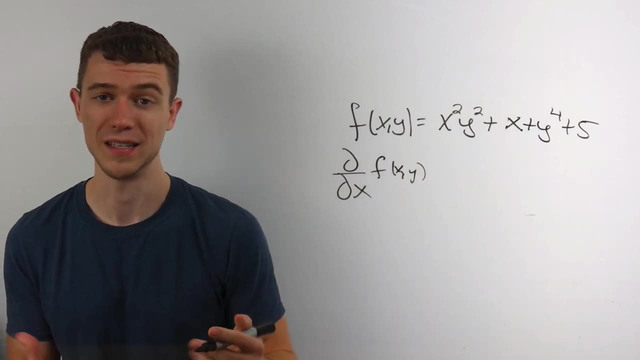 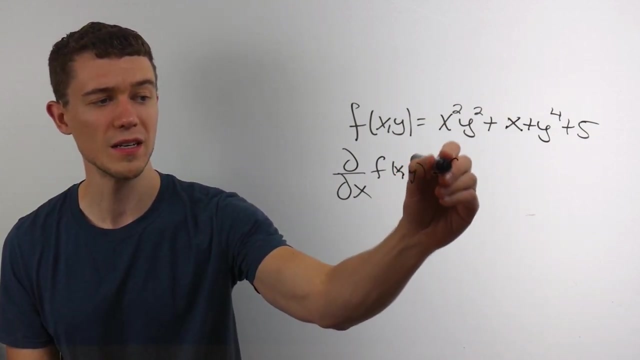 x and y, a two variable function. we could take the partial derivative with respect to x of this function And this is the notation that you might see this curly backwards d thing. this signifies partial derivatives. You might also see f sub little x. this is also a notation for partial 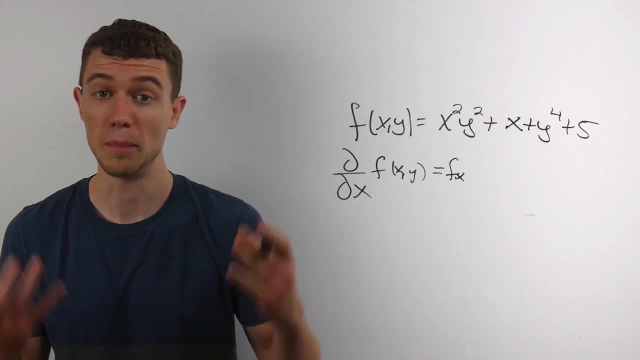 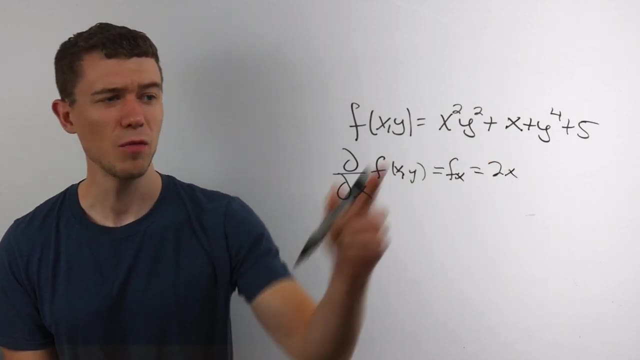 derivatives. But let's do it. we really just have to remember the power rule for derivatives here. What's the derivative of x squared? Well, it's 2x, right. And what about the y squared? Well, we just leave it, because derivatives 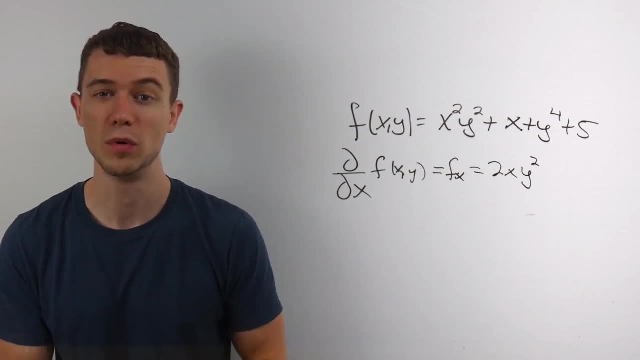 keep constants. constants stay along for the ride when we're taking derivatives, and the partial with respect to x, y is a constant here. What about the derivative of x? Well, the derivative of x with respect to x is still 1, right. What about y to the fourth? Well, the derivative 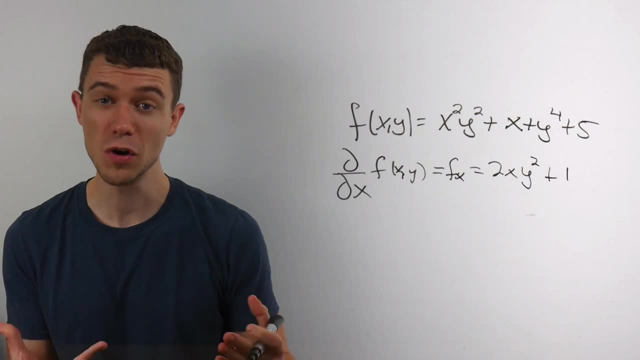 of y to the fourth, with respect to x, is 0,. right, y is a constant. here the derivative of a constant is 0.. Same with this: 5,. right, The derivative of 5 is 0,. so that's it. That's the entire partial derivative. 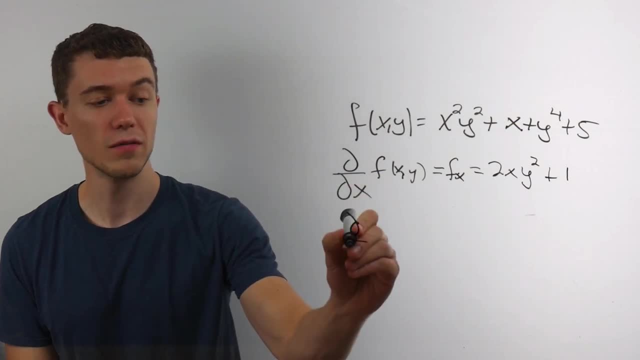 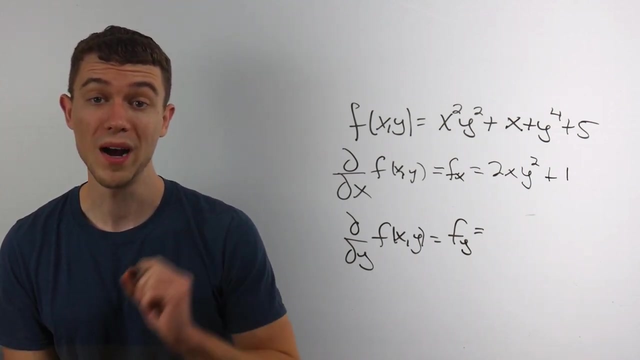 It's actually not too bad. We can do the partial derivative of this function with respect to y as well. You might see it denoted like this or like this: the f sub y. These mean the same thing. Let's do it. let's take the partial derivative with respect to y this time, meaning x is a. 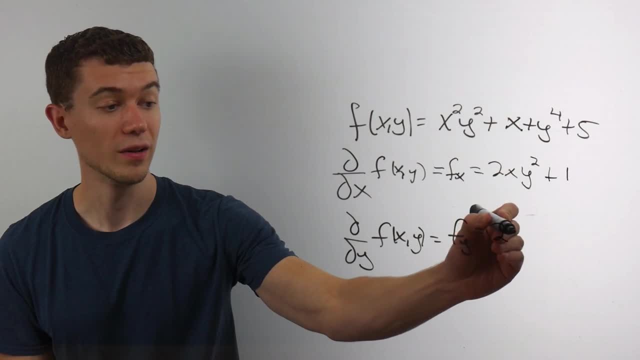 constant. So what's the derivative of y squared? Well, it's 2x, right? And what about the partial derivative of y squared? Well, again, it's 2y, and I'll keep the x squared, just pretending it's. 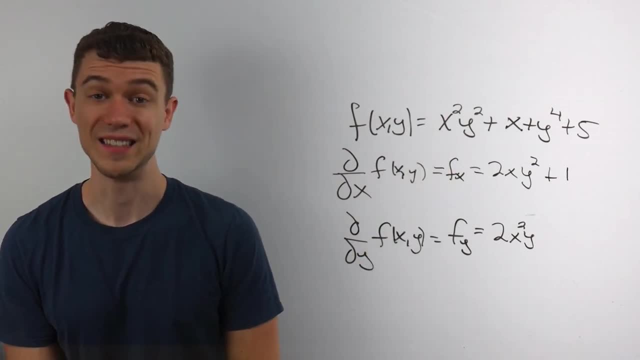 like a constant, The derivative of x is 0,. because x is now a constant, The derivative of y to the fourth would be 4y cubed, just like you would expect from the power rule, and the derivative of 5 is 0..